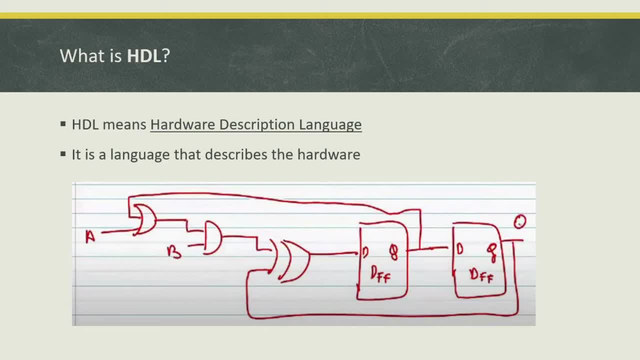 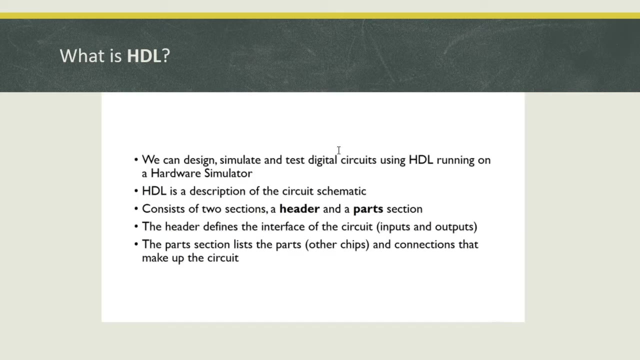 We will have a hard time to draw 10 times more of this Now. it's not scalable. It's not scalable. So that's why HDL is very important. Now we can design, simulate and test digital circuits using HDL, running on a simulator, of course. 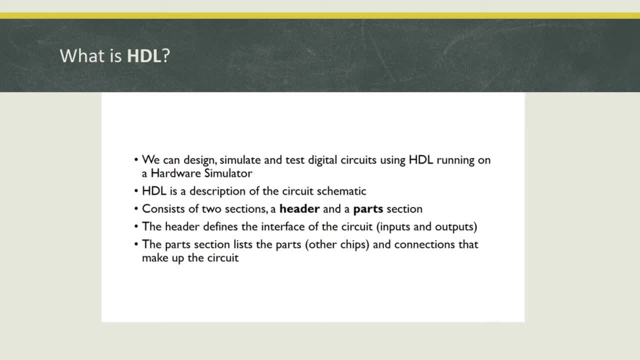 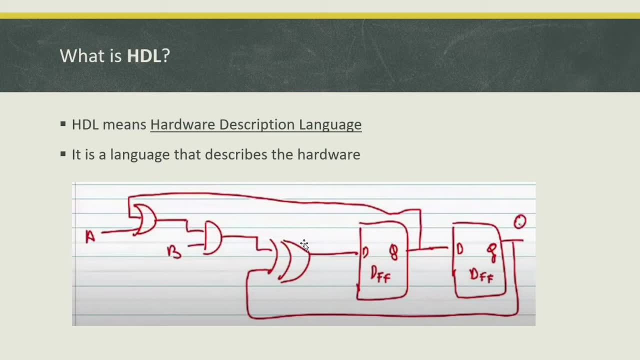 It is a description of the circuit schematic. So description of a circuit schematic, for example. here you can see what is the description of this. This is the first study, So it consists of two sections. We have header and parts. 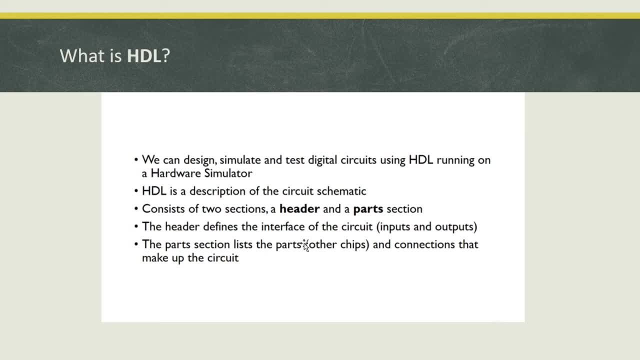 So header, it defines the interface of the circuit. So obviously, in making a digital circuit or in making a circuit, we have inputs right. For example, in our IC which is 74LS08, it has inputs, it has outputs. 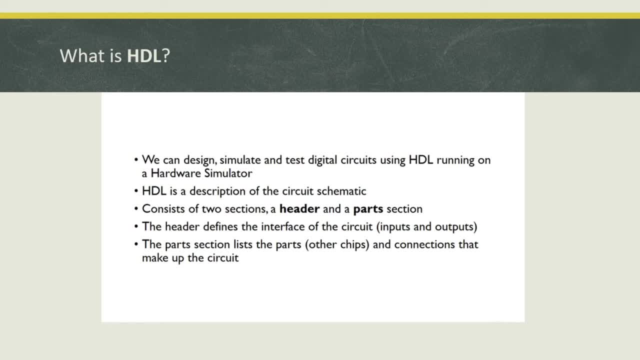 So the output, you put it in the input in the PCAS IC. So it has that. So those defines the header. So it's just part of the header. in HDL Now we also have the parts section. So the parts sections are other chips and connections that make up the circuit. 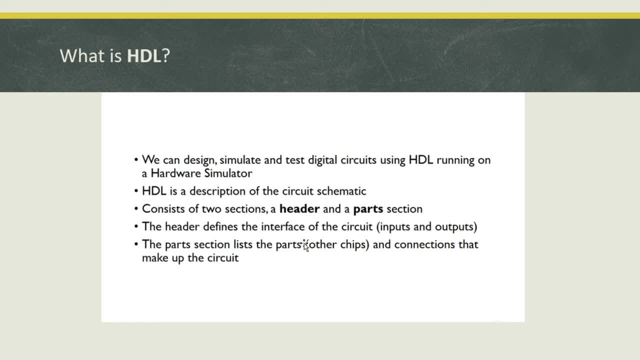 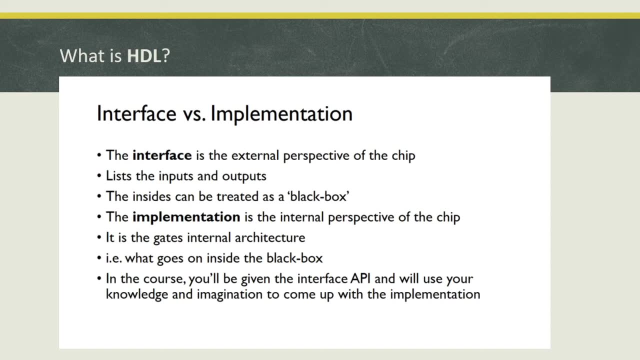 So, like wires, it has other parts in the parts section. Now let's talk about the interface and the implementation. Okay, in HDL we will see interface and implementation in totality as a whole. So for example, For interface it's the external perspective of the chip. 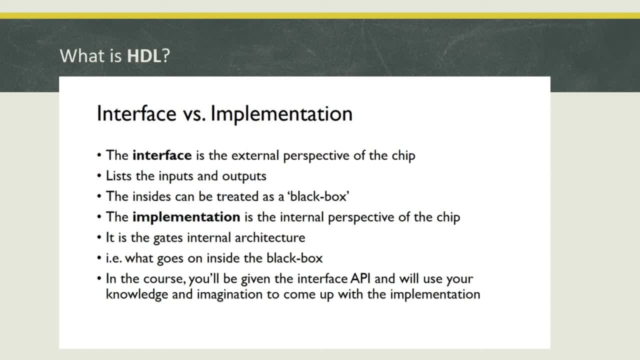 Okay, what you see is only in the circuit, For example, NE555 timer. If this is in the circuit of the NE555 timer, this is the interface. So we won't see the sequence in the NE555, because that would now be the implementation. 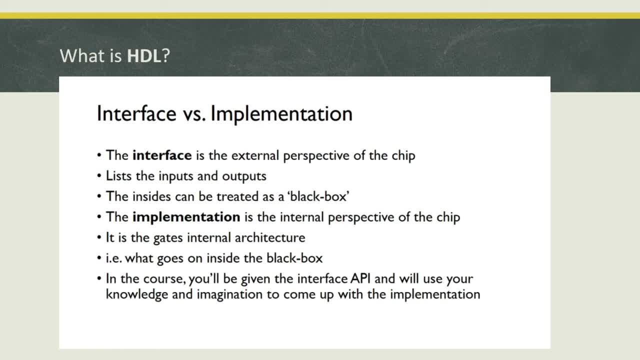 So the interface lists the input and outputs. So input and output only. We can see that this is just the output And the insides can be treated as a black box. Now the implementation is the internal perspective of the chip. 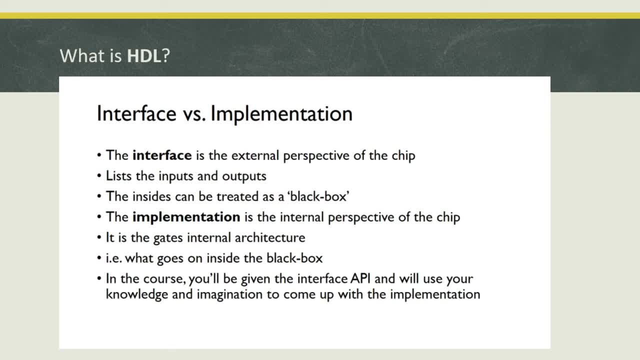 So if the chip is connected to your chip- for example again another IC NE555, if it's connected to the NE555, it's a pulse right, So because it's a timer, So it's the gates. internal architecture. 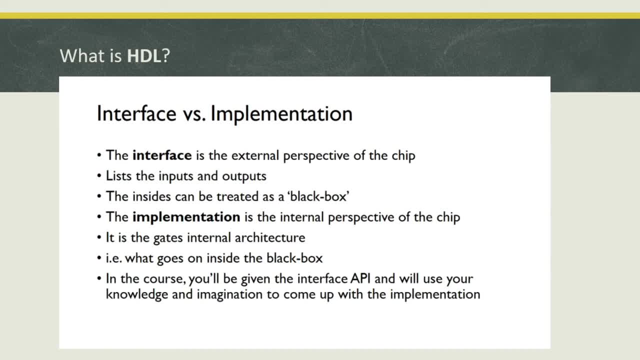 So it's the gates internal architecture. So it's the gates internal architecture. It goes on inside the black box. Let me think of an example. It looks like a computer where it has an interface and a monitor, But we do not know what's going on inside it. 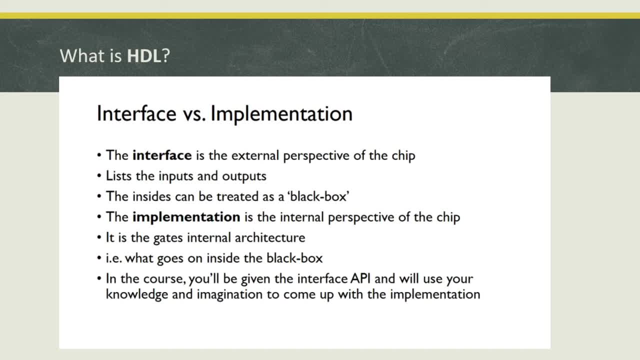 There's an operating system that is working on the data. There's an ICPU that processes the data. So it's the same here in HDL, But we're just talking about the creation of an integrated circuit. Okay So, or the designing of an integrated circuit. 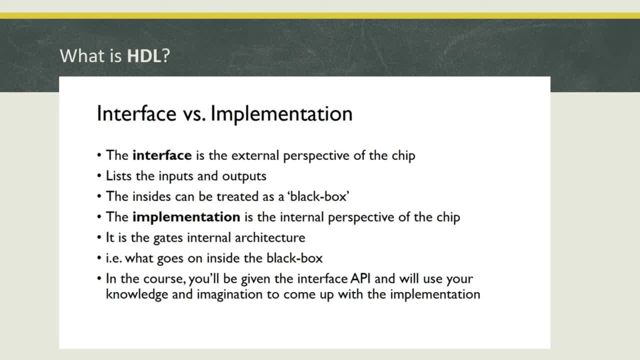 So in this course you'll be given the interface API and will use your knowledge and imagination to come up with the implementation. So API just means the Application Programming Interface. It's a software intermediary that allows two applications to talk to each other. Okay, 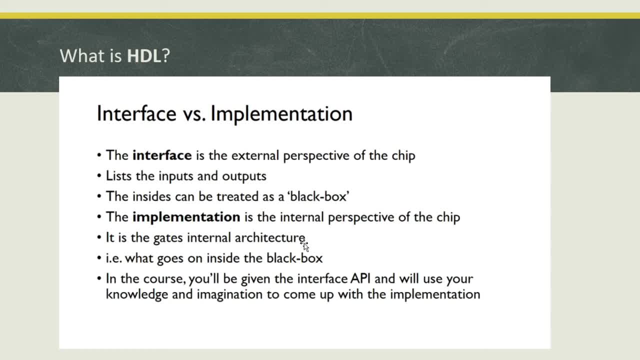 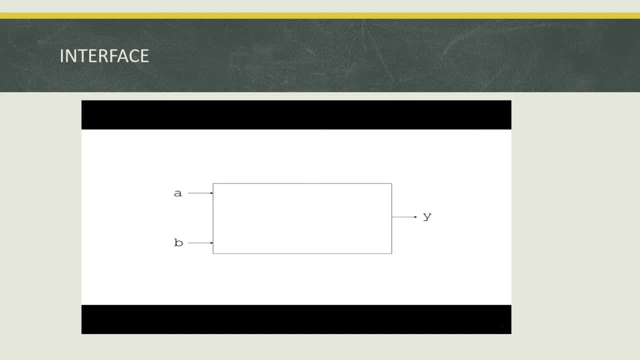 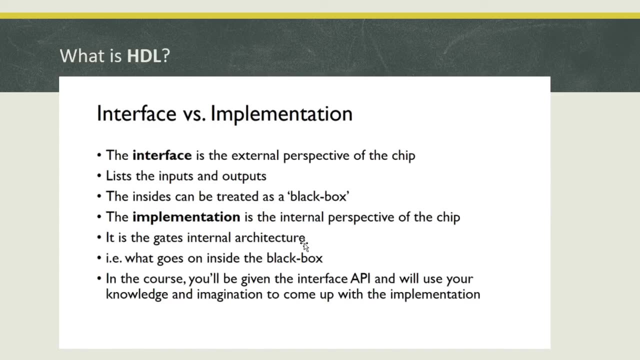 Now to further match the interface versus implementation, let's look at this circuit Now. this is just an interface, because what we see is a circuit As described earlier. it just gives the lists of inputs and outputs. It's just internal perspective of the chip. 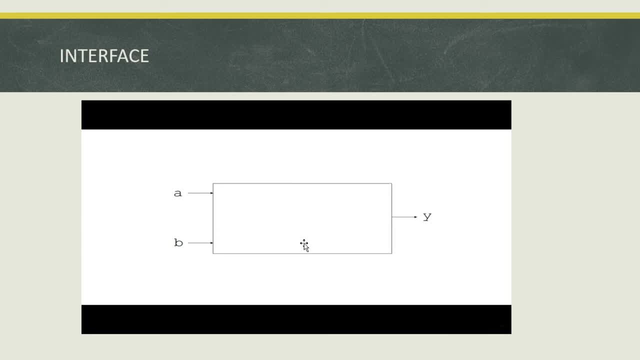 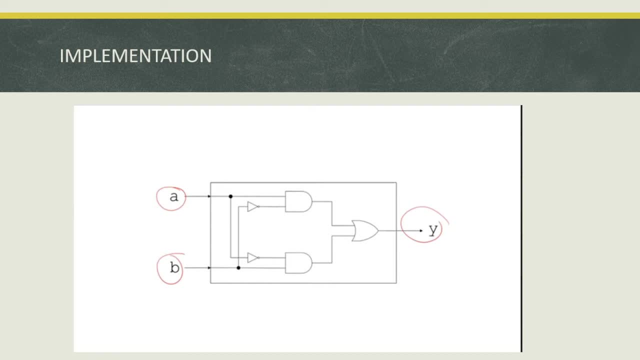 It's just a circuit. It looks like it. So input and output, But the implementation is what we don't see inside the interface. So it's not implemented in the previous integrated circuit. Okay, So I hope you understood the difference between the two.